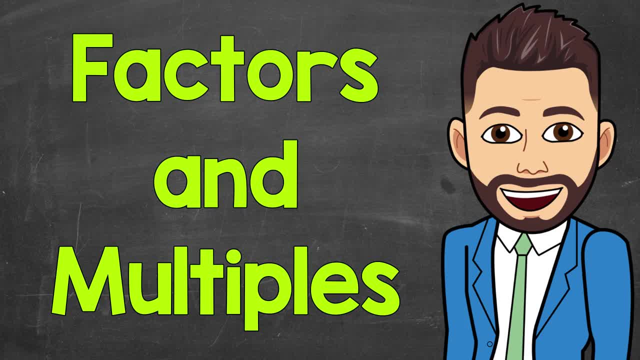 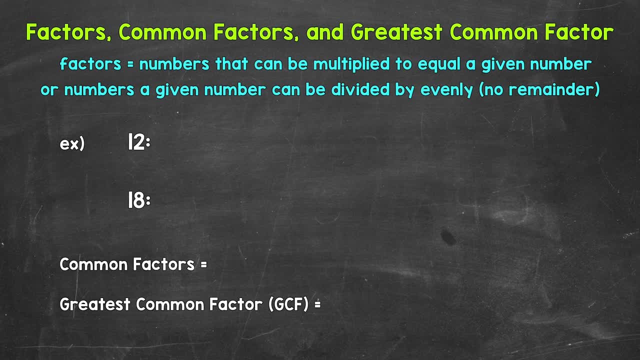 Welcome to Math with Mr J. In this video I'm going to cover factors and multiples, common factors and multiples, and then greatest common factor and least common multiple. We're going to start with factors, common factors and greatest common factor and then go from there. 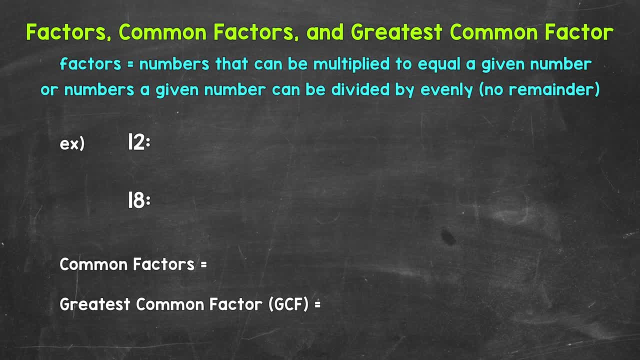 Now, when we think of factors of a number, we need to think what numbers can we multiply to equal that given number? Or what numbers can we divide that given number by evenly, So divide with no remainder. Now, it's not the most technical, or? 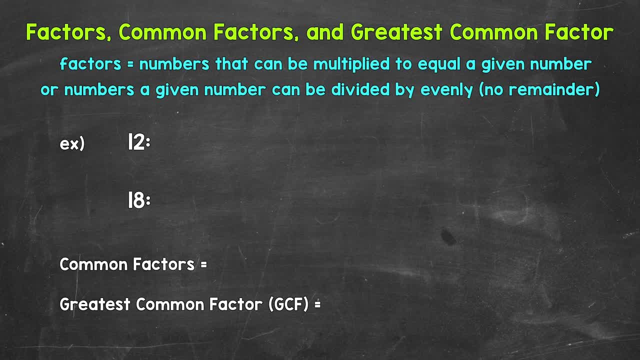 mathematical way to word it, but you can think what numbers go into the given number. This will all make a lot more sense as we go through our example. Let's jump into our example where we have a number that is equal to a given number. We're going to start with a number that is equal. 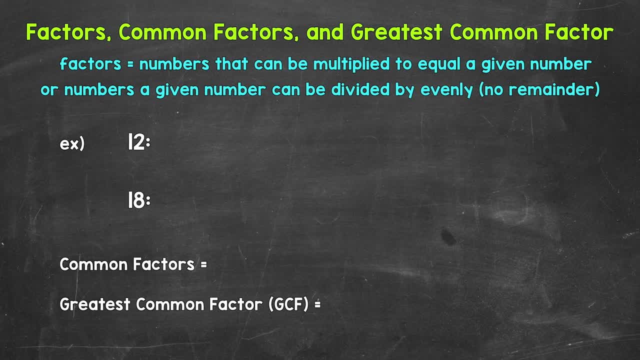 to a given number. We're going to start with a number that is equal to a given number. We're going to list the factors of 12 and 18, then find common factors and then, lastly, find the greatest common factor, which is also referred to as the GCF. Let's start with the factors of 12.. And my 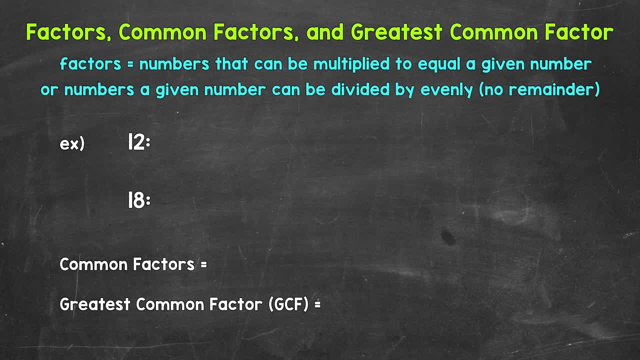 suggestion would be to always start with 1 and the number itself. We can think of factors in terms of pairs, We can think of factors in terms of numbers and we can think of factors in terms of numbers. So 1 times 12 equals 12, or we can divide 12 by those factors, however you want. 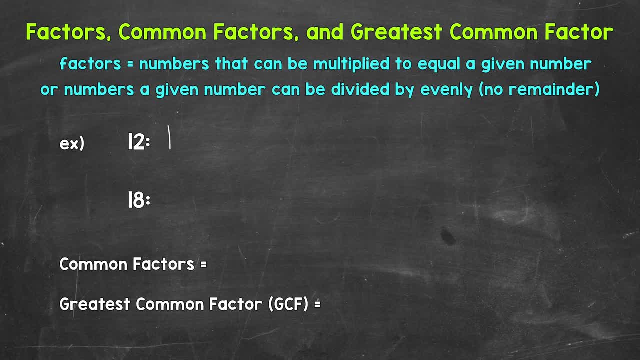 to think about it. So I'm going to write 1 and 12 with a gap in between. That way, we can write the other factors in between 1 and 12, and we can write them in order. Now we need to list the other factors of 12.. So let's think about what else goes into the. 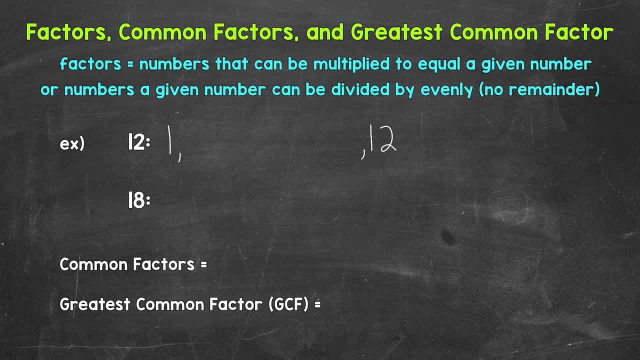 12,, so to speak. Think of multiplication facts, division facts, and we can work our way up from 1.. So there are different strategies and ways to work through this. The next factors are 2 and 6.. 2 times 6 equals 12.. So 2 and 6 are factors of 12.. So 2 and 6.. Then we have 3 and 4.. 3 times 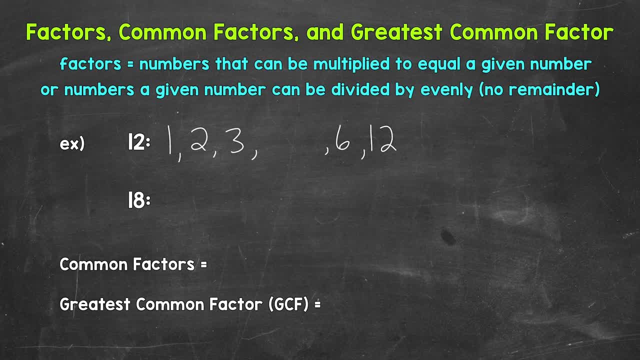 4 equals 12. So 2 and 6 are factors of 12.. So 2 and 6.. Then we have 3 and 4.. 3 times 4 equals 12.. So 3 and 4 are factors of 12 as well. And again we can also think of these factors in. 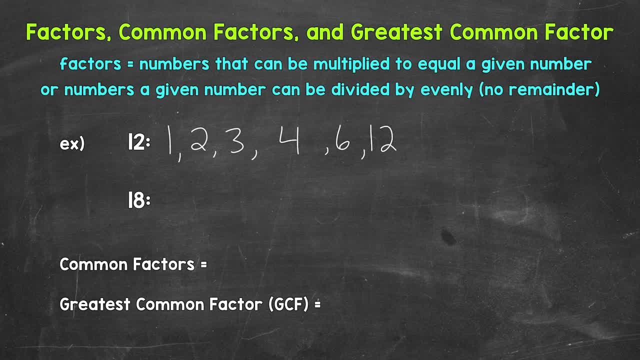 terms of division. We can divide 12 evenly by these factors. Now, are there any more factors of 12?? No, We are done. That's our list of factors for 12.. Let's move on to the factors of 18.. We. 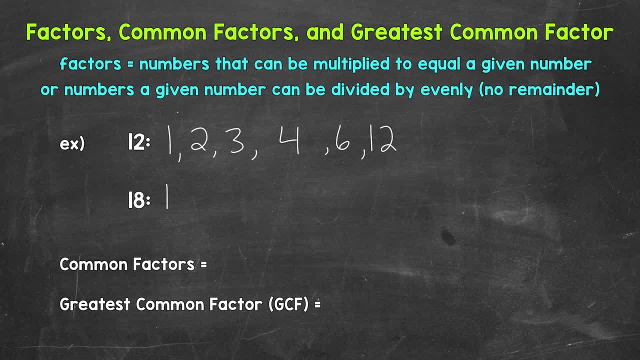 will start with 1 and 18.. So 1 and 18, with a gap in between. Next we have 2 and 9.. 2 times 9 equals 18.. So 2 and 9 are factors. Then we have 3 and 6.. 3 times 6 equals 18.. So 3 and 6 are factors of 18.. And that's it. 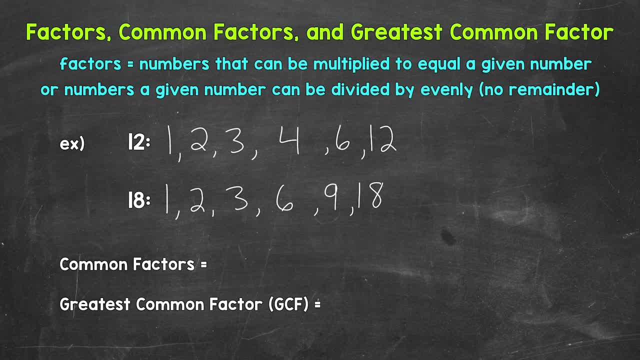 for the factors of 18.. You can always try to figure out the factors of 18.. You can always try to figure out the factors of 18.. You can always try to figure out the factors of 18.. You can always try more if you're unsure. if you have all of the factors, For example, we can think about 4,, 5,. 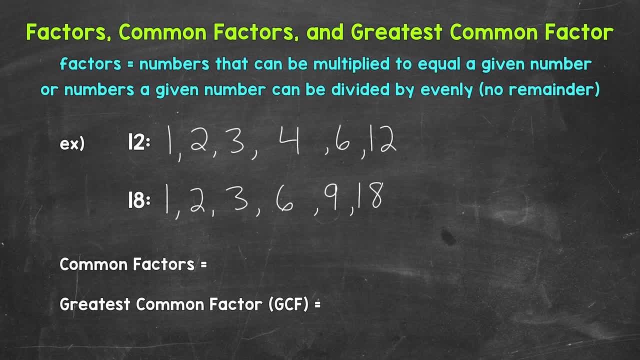 7,, 8, and so on. But we are done. That's our list of factors for 18.. One thing I do want to mention about factors and writing out these factor lists is that you will get better the more you do So. 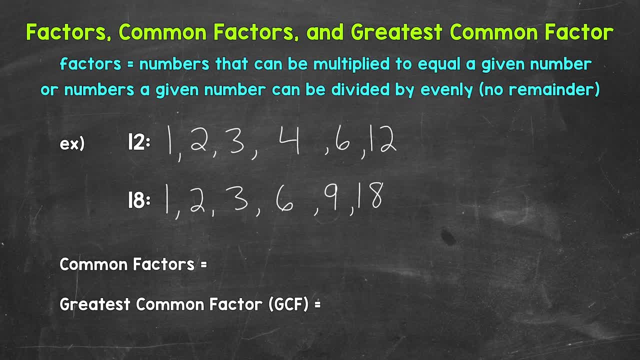 writing the factors, the spacing of your lists or whatever else the case may be. So something to keep in mind. Now let's take a look at the common factors between 12 and 18.. That just means the factors they share, The factors they have in common. So 1 is a common factor, 2 is a common. 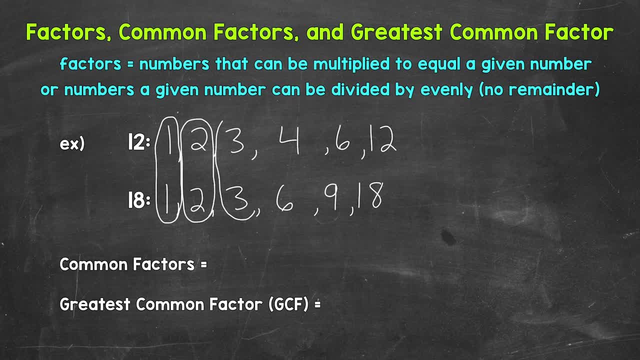 factor. 3 is a common factor And then 6 is a common factor. So the common factors between 12- 18 are 1,, 2,, 3, and 6.. Now we have the greatest common factor, or GCF. That's just the greatest. 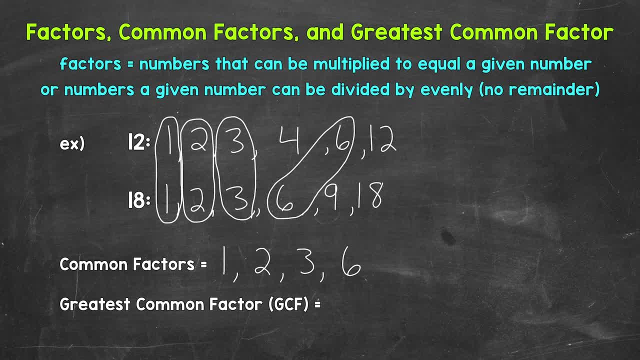 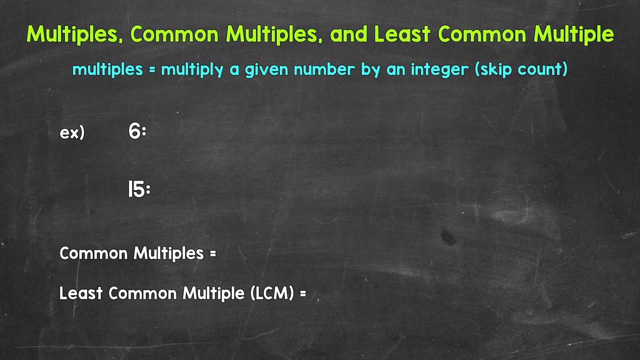 factor in value that they share or have in common. The greatest common factor between 12 and 18 is 6.. So the greatest common factor equals 6.. So there's an explanation of factors, common factors and greatest common factor. Let's move on Now. let's take a look at multiples, common multiples. 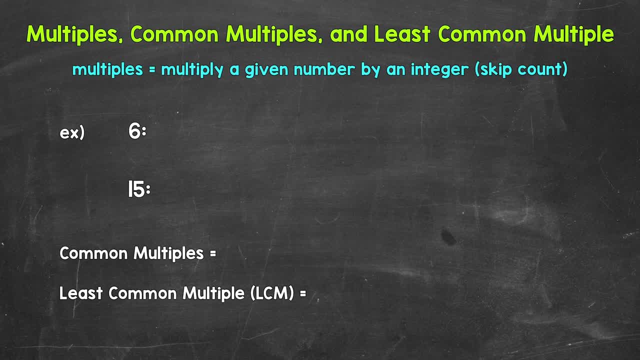 and least common multiple. Now, a multiple is the result of multiplying a given number by an integer. So when we think of a given number, we think of a given number as a given number. When we think of the multiples of a number, we need to think about the numbers we get when. 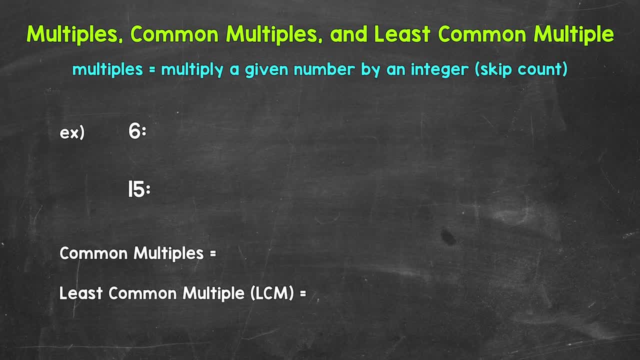 multiplying that given number by integers. A simpler way to think about multiples is to think about skip counting. So all of the numbers, something is going to hit when you count up by that number. those are all going to be multiples. This will make a lot more sense. 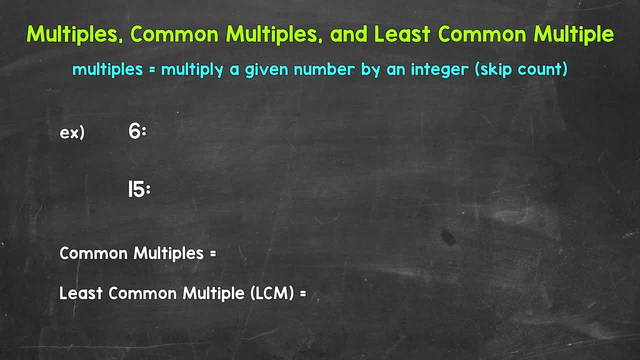 as we go through our example. Let's jump into our example where we have a number that is a given number. We have a number that is a given number. We have 6 and 15.. We're going to list some multiples of 6 and 15, look at common multiples. 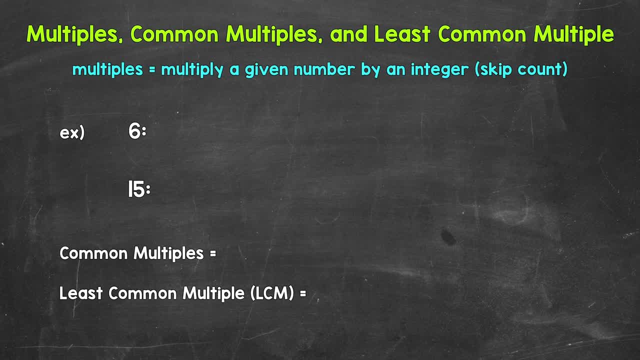 and then find the least common multiple, also referred to as the LCM. Let's start with the first five multiples of 6, which are 6 times 1,, which is 6.. 6 times 2 is 12.. 6 times 3,. 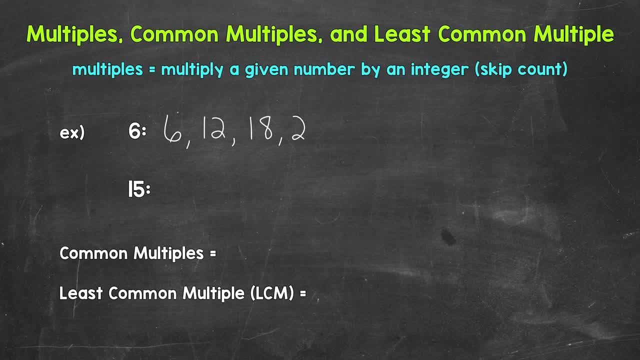 is 18.. 6 times 4, is 24.. And 6 times 5, is 30. So those are the first five multiples of 6.. And you can see that we just skip counted by 6.. 6,, 12,, 18,, 24,, 30,, so on and so forth. 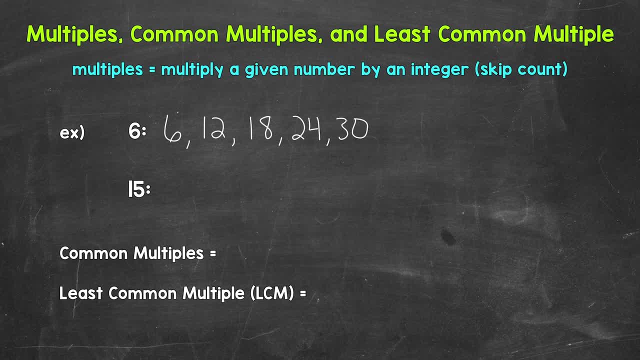 Now I stopped at 30 because multiples go on forever, They are endless, They are infinite. My suggestion is to list four or five multiples when looking for common multiples or the least common multiple. So list four or five, Look for any in common And if you don't have any in common, 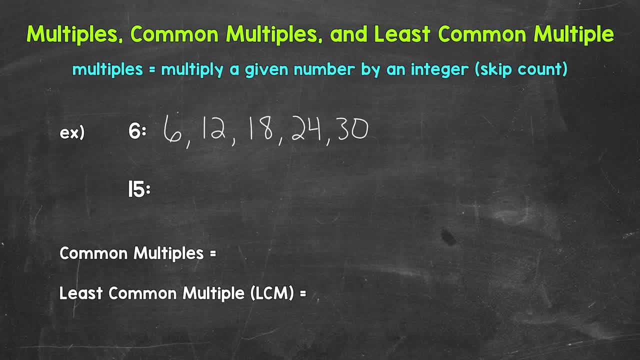 you can always extend the multiples lists. Now let's list the first five: multiples of 15.. So 15 times 1 is 15.. 15 times 2 is 30.. 15 times 3 is 45.. 15 times 4 is 60. And then 15 times 5 is 75.. 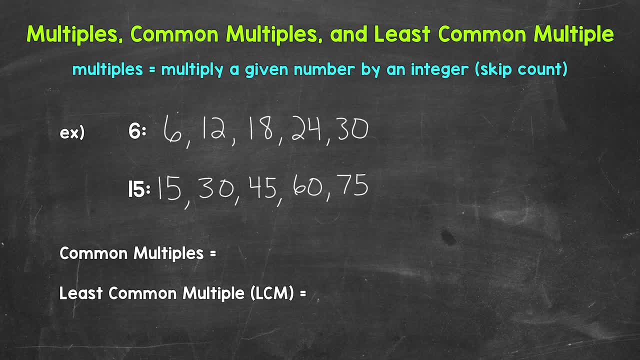 Now let's look for any common multiples, So any multiples they share, any multiples they have in common. Well, 30 is a common multiple. The next common multiple is 6.. The next common multiple is 60. So let's extend the list of multiples for 6 there to show another. 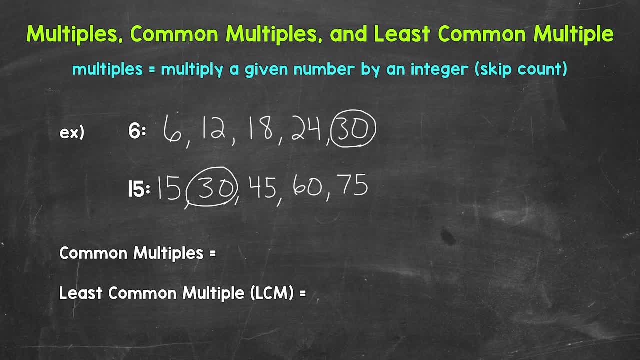 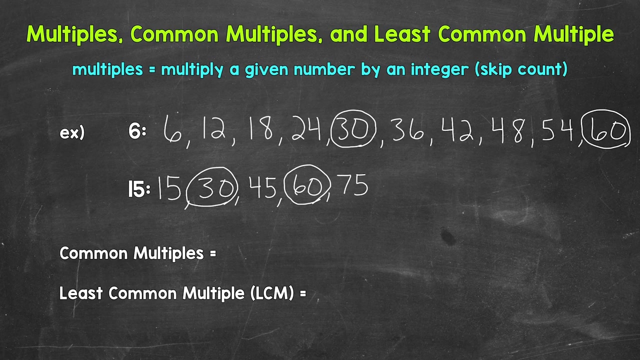 common multiple. So after 30, we have 36., Then 42., Then 48., Then 54., Then 60. So another common multiple is 60. But again, remember, multiples lists go on forever. So we have an infinite amount of common multiples. 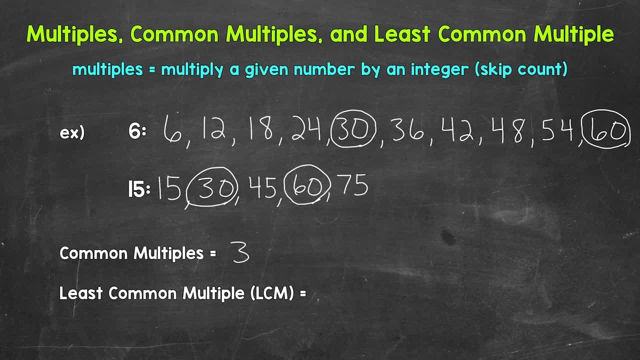 So down below for common multiples, I'll put 30,, 60, and then make note that we have an infinite amount of common multiples. Now we have the least common multiple, which is just the smallest number in value that they have in common, The smallest number in value that they share. This is going to be 30.. 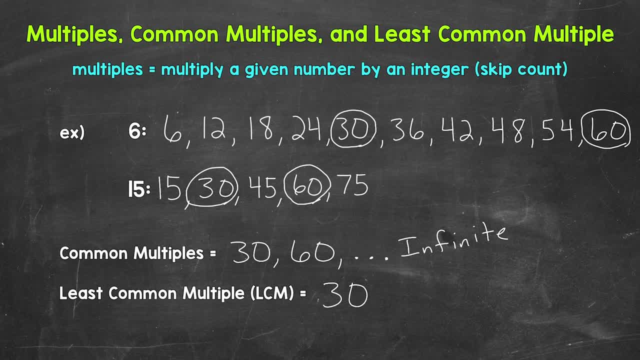 The least common multiple, or LCM, between 6 and 15 is 30.. So there you have it. There's an explanation of multiples, common multiples and least common multiple, along with the explanation of factors, common factors and greatest common factors.